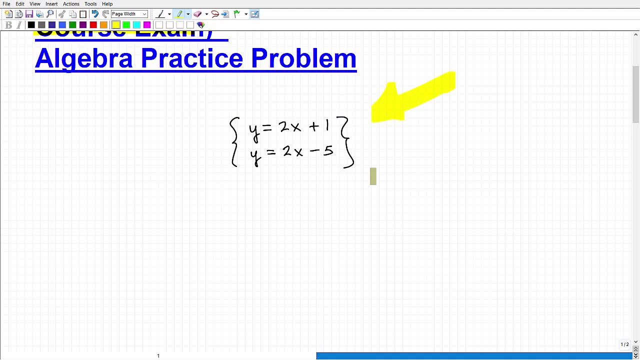 And I'd like you to solve this. Okay, Solve this. So you might want to go and pause the video and do so Now. for those of you that are not quite sure, I'm going to give you now a hint, Okay. So if you don't want to hear the hint, pause the video, But if you need a little bit of a hint before I fully solve it, this is the hint, Okay. So what are we talking about here? Well, we're talking about a system. All right, A system of equations is a big topic in algebra. 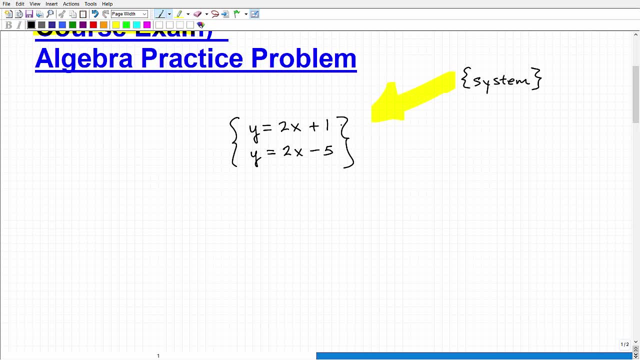 Algebra one: Okay, Linear systems actually. So I want you to solve for X and Y, Okay, X and Y, Now a little bit more of a clue, Okay. So of course, if you don't want to hear this, you know. if you figure you could solve this problem on your own, do so Okay. But in algebra one you learn various strategies on how to solve systems- linear systems: Okay, There's techniques and they're extremely 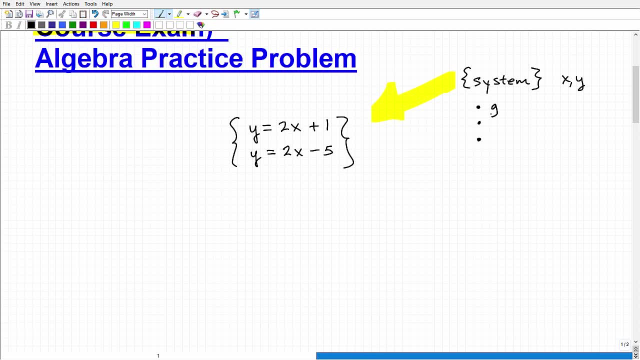 important for you to know. So the first would be like the graphing method. Okay, And I'm not going to fully explain this to you And I don't want to turn this into a full lesson on systems, as this is a huge topic. Then you would have the substitution method and or the linear combination or elimination method. So you need to know all three, But conceptually, you need to know what a system represents, Okay, And then, of course, how to solve systems. So now, hopefully, all of this kind of 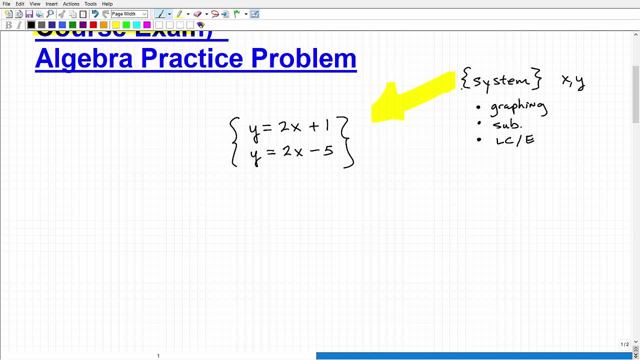 has jogged your memory and you're like, oh, okay, I remember this stuff. Now I know how to solve this, So go ahead and solve it. if you know how to. Okay, So let's get to the solution. Okay, Now, first of all, I'm going to solve this without actually even doing any work. Okay, You're going to say, well, like, how's that going to work? Well, I'll show you this in a second. Well, first of all, we have to understand what are we talking about. 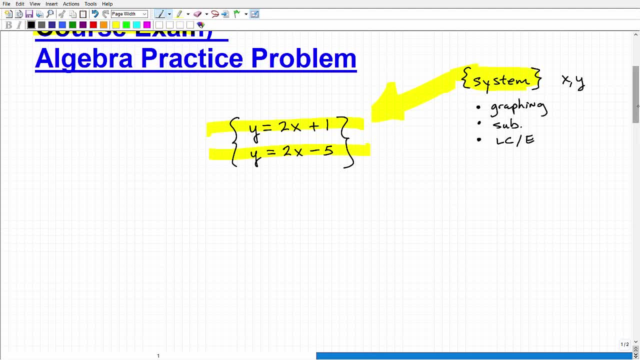 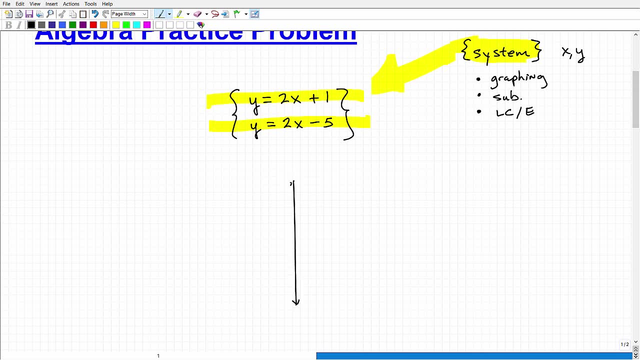 Well, we're discussing systems. Well, systems, Okay, Graphically speaking, systems are basically two lines, Okay, On the X- Y axis. So let me just quickly just do a little sketch here. So here's X and here's Y. So we would have maybe one line like so line one, And then maybe another line like this: This would be like line two And the intersection, Okay, Where these two lines cross. 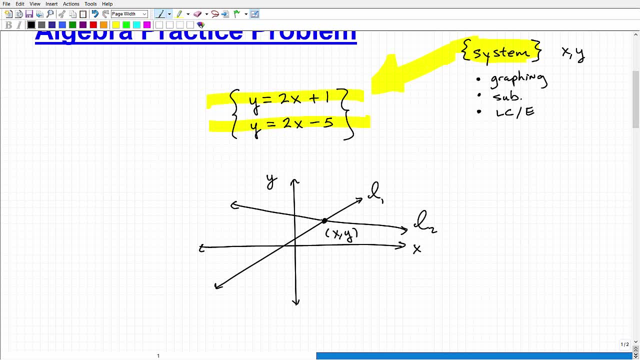 Is a particular coordinate, an order pair, right, An X- Y point on the X- Y plane. Okay, Now, this X- Y, where this particular point is graphically how we interpret the solution to a system. Okay, So when you're trying to solve systems, you can think of this as a line. Okay, This is one line and this is another line. And if I was to graph them and then look and see, hey, where those lines cross, that would be an illustration. 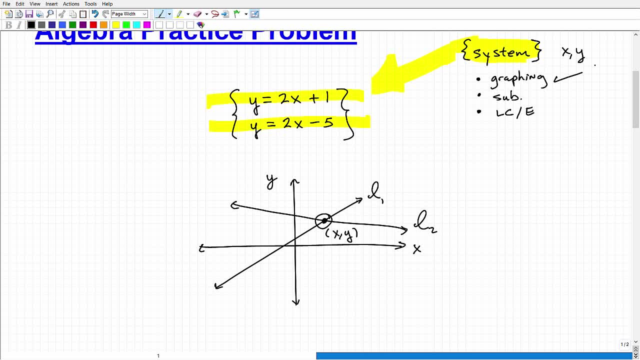 Of the graphing method, But that's visually or graphically, what's going on with the system. Now, again, I don't want to make this problem you know too long and turn it into a full lesson on systems. Okay, This is a big topic and something you need to know. Of course, I teach all of this and more in my prep course, But let's kind of get to the what's going on here now. Okay, Now, if I'm looking at this, I have some sort of line. Okay, Now, this is the line. 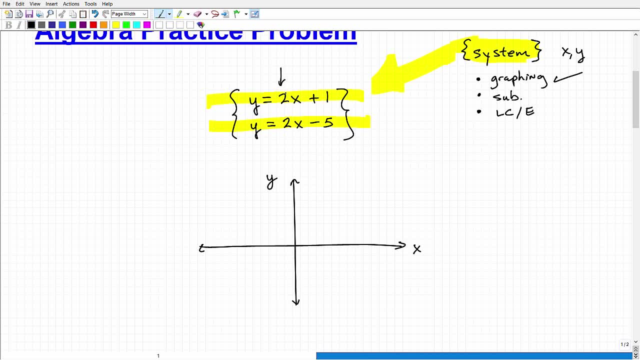 The line Y equals 2X plus 1.. So it has a slope of 2.. Okay, And a Y intercept of 1.. So it would maybe go through, or it is going to go through, the Y axis at 1., Okay, And have a slope of 2.. So maybe something- Oops, That's not good, Maybe something like that. Okay Would be, let's call this line 1.. Now let's take a look at the second line. Okay, This second line also has a slope of 2. But it has a different slope. 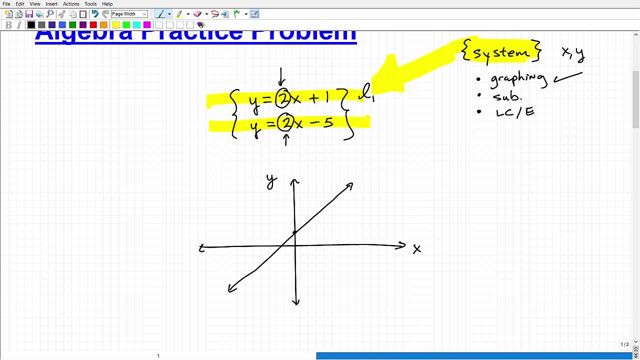 It has a different Y intercept. So what does that mean to you, Okay? Well, hopefully you're saying: oh, this line, Okay, Is parallel, All right, This is going to go through. this first line is going to go through the Y axis at 1.. And the second line is going to go through the Y axis at negative 5.. So here's line 2.. Here's line 1., Here's line 2.. So the situation is what? Well, these lines are parallel. They're never going to cross. Okay, So what does that mean? Well, if lines never cross, 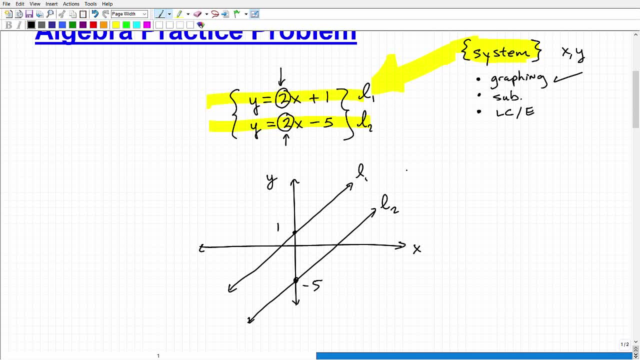 when we're talking about learning your systems, there is no solution. So here, the answer is no solution, Okay, So the way you could have seen this is: just notice that, hey, we're dealing with two lines. They have the same slope, a different Y intercept, Excuse me, So there would be no solution. Okay, So let's go ahead and actually do a little bit more work. 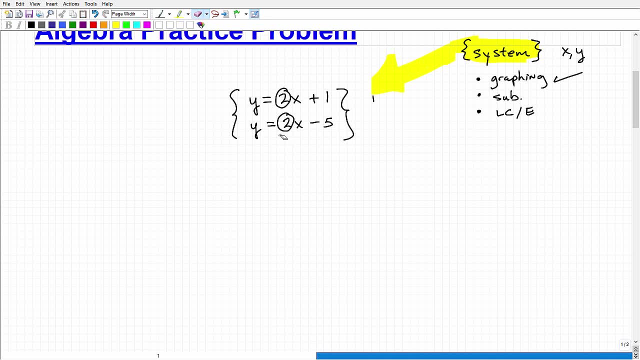 All right, And let's say, algebraically, we wanted to see what was going on So we could use the substitution method. So I have: Y is equal to 2X minus 5.. So I'll replace this Y with this stuff right here, So you can use a substitution method. So I'll replace this Y with this. Okay, So that's going to be: 2X minus 5 is equal to 2X plus 1.. 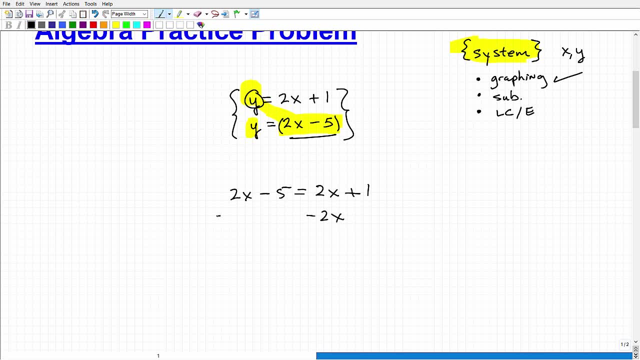 Now, if I solve for X, what's going to happen here? Okay, Well, I'm subtract 2X from both sides of the equation and I end up with 0.. Okay, Minus 5 equals 1, or negative 5 is equal to 1.. And that makes no sense. Okay, You're like what's going on? This is a false statement. So when you get a situation where the left is not equal to the right, Okay, When you're trying to solve a system, that's an indication that there is no solution.